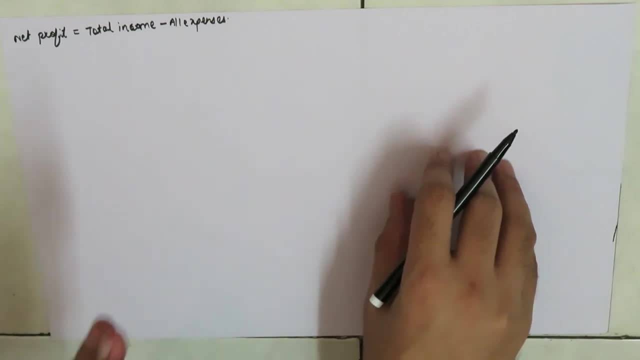 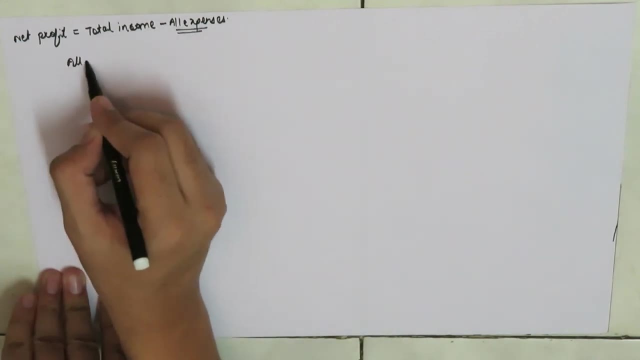 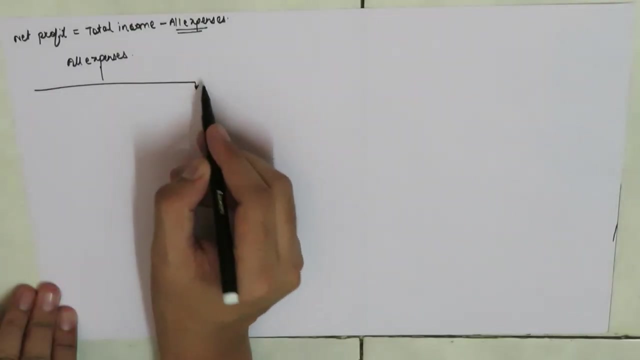 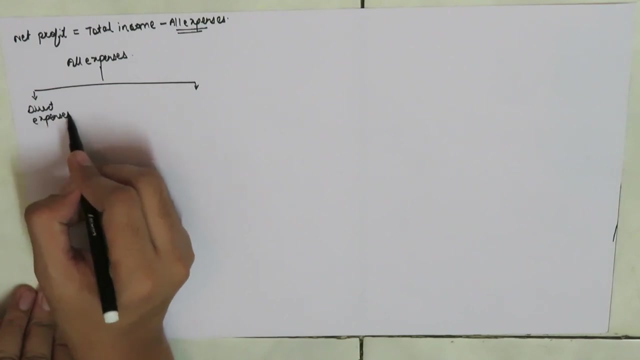 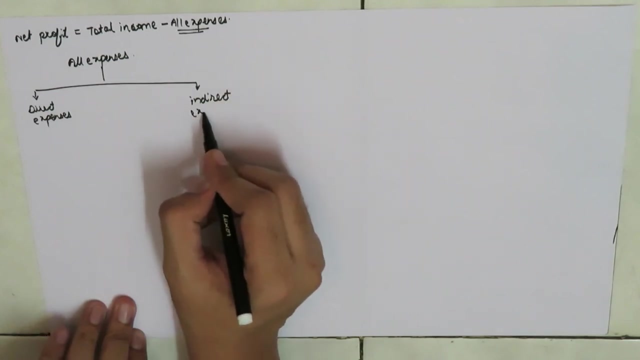 be aware of the many different types of cost involved in a manufacturing processes. so in this case, this all expenses is again divided into two parts. this all expenses is again divided into two parts, that is, the direct expenses and another one is indirect expenses. so in the case of the 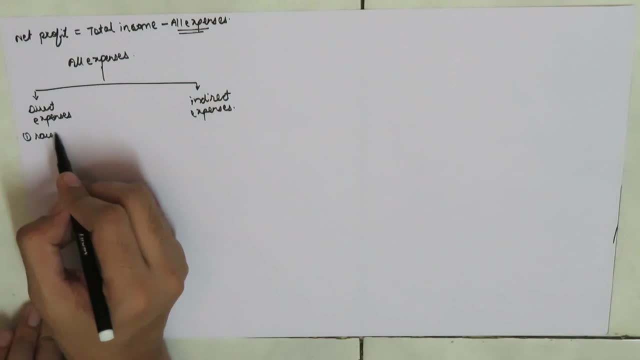 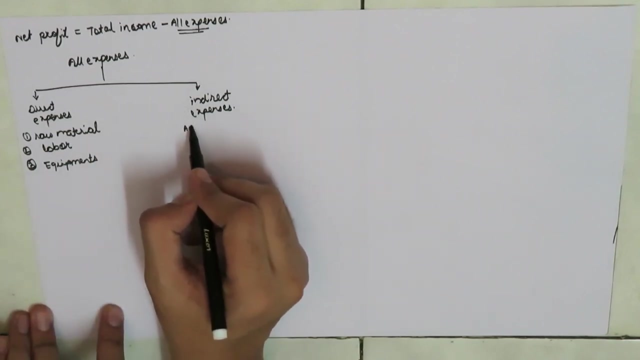 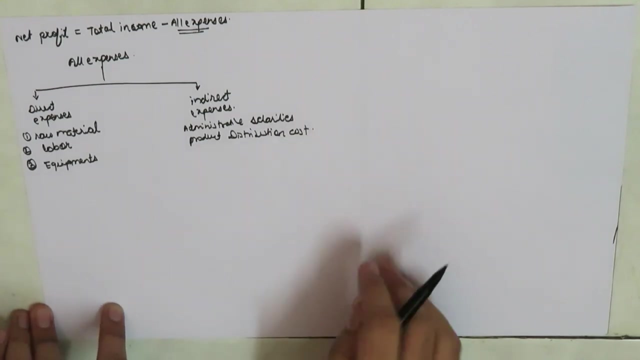 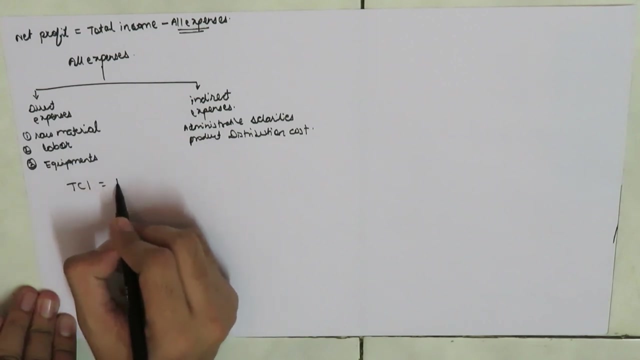 direct expenses. we need to manage the raw material expense for the plant and we need to manage the labor, we need to manage equipments in the plant. and in the case of the indirect expenses, these expenses include the administrative salaries, administrative salaries and the product distribution cost and in this case we know that our total capital investment is equal to the fixed capital. 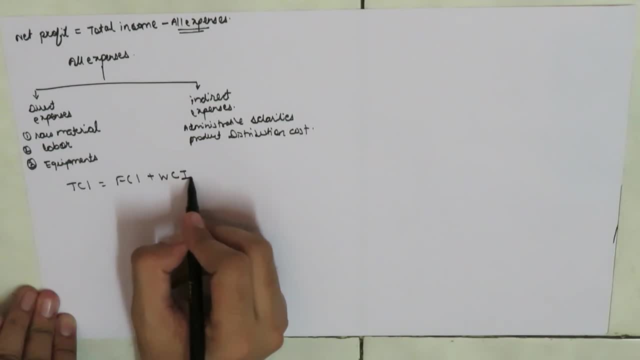 investment plus the working capital investment, and in this case the fixed capital investment is used for the physical equipment facilities. so this is mainly used for the physical equipment facilities. so this is mainly used for the physical equipment facilities and this working capital investment can, and this working capital investment can. 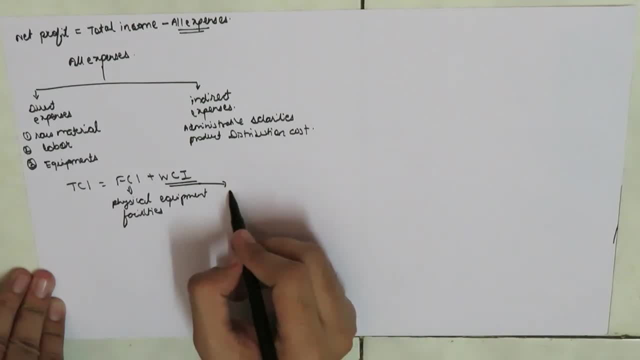 be used to keep the raw materials and products in hand. to keep the raw materials people. the very classic example of keeping the raw materials in is to keep the raw materials and products and products in hand. the very classic example of keeping the raw materials in hand is in. 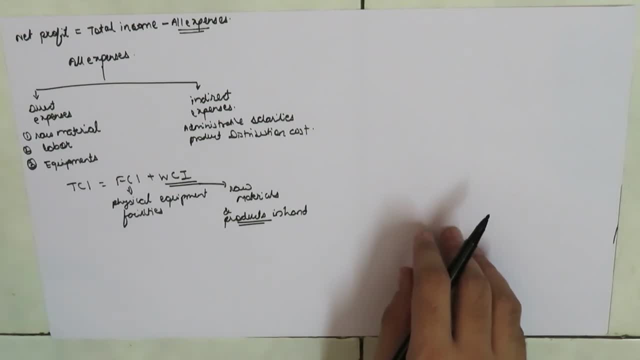 the case of the dairy industry's, where the cheese once produced is kept in hand, where the cheese once produced is kept for the cheese curing, or which is also called as the cheese maturation, and in this case the cheese is kept or stored in the dairy for about six to seven months to improve the texture, to improve. 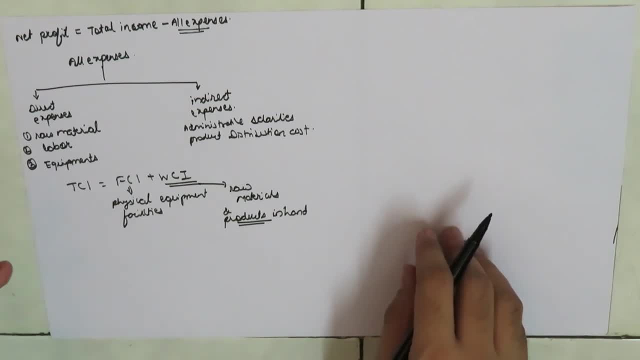 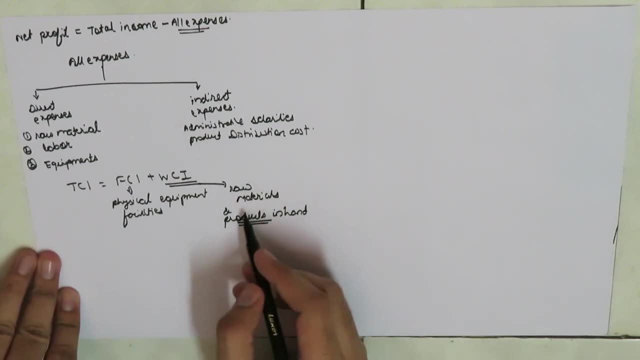 the taste of the cheese, and in order to store this cheese, we need to build a storage block. so when we build a storage block in the dairy industry, the wrong, the material which is produced- needs some expenses. okay, so, without wasting our time, we are going to solve some of the classic. 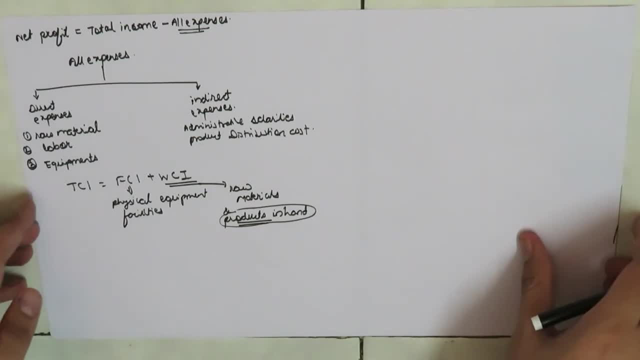 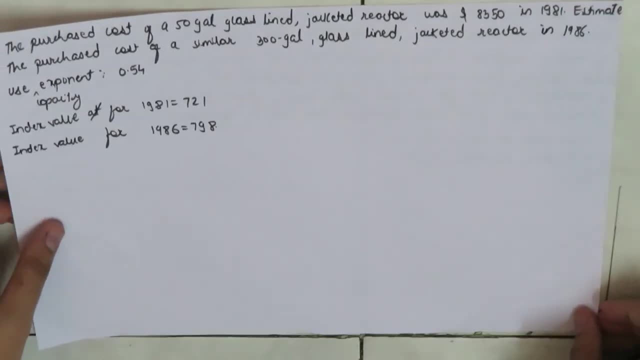 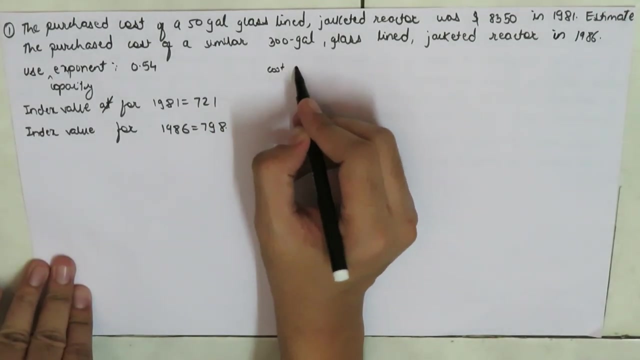 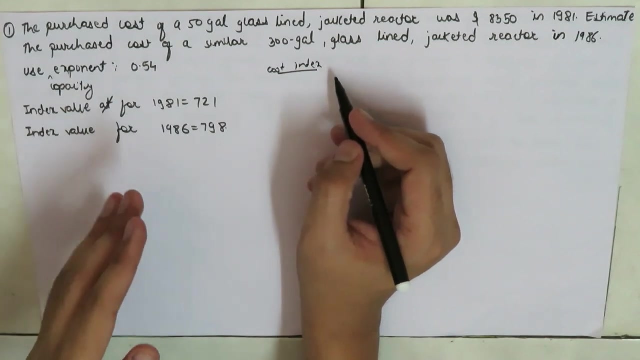 examples which are dependent upon the cost estimation. so here is the first example, and before they are directly putting hand with the example, I like to introduce the term which is called the cost index. so in the case of the cost index, it is nearly an index value for given in time, showing the cost of that time relative to the 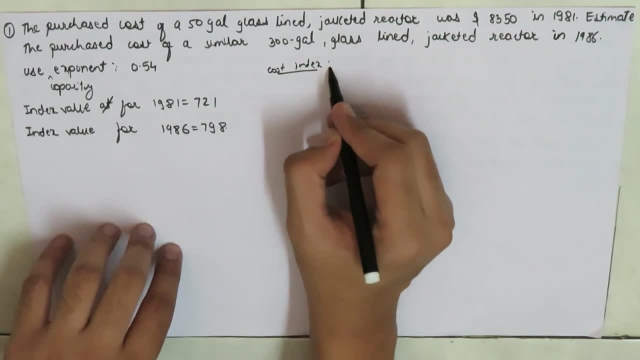 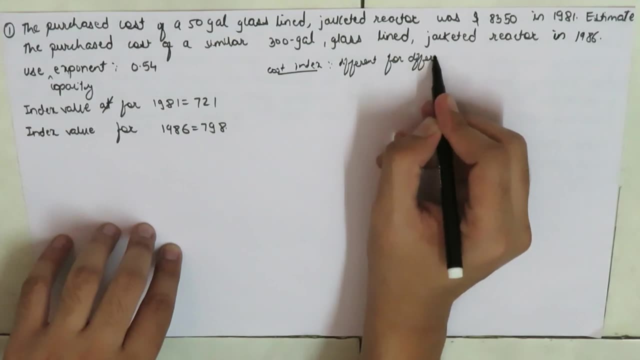 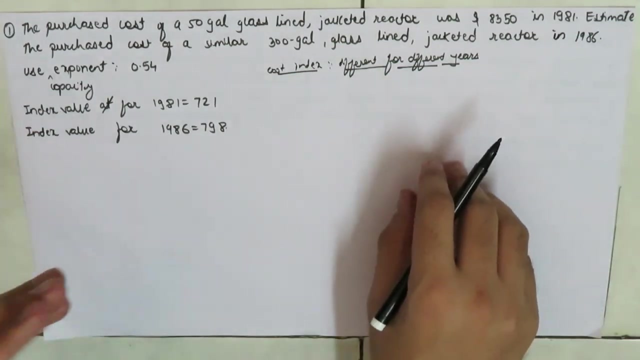 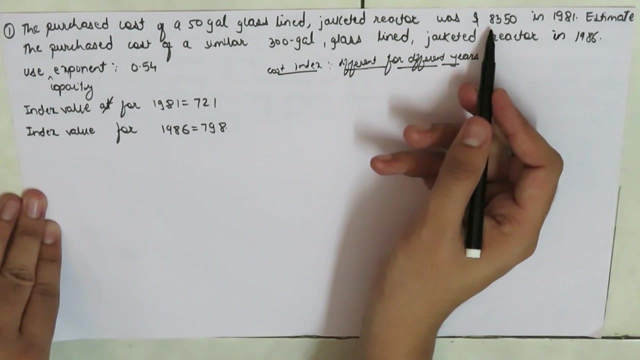 certain base time means the cost index is different for different years. so in order to get a deep understanding of this Cost Index, let's Information example which is dependent upon the cost index. here we have our question. the purchased cost of the 50 gallon glass line jacketed reactor was $8,350 in 1981 and estimate the purchased cost of the. similar 300 gallon reactor- jagged reactor- in 1986 and by making the use of the capacity exponent as 0.54 and the index value in the case of the year 1981 is $7.21 and the index value for 1986 is $7.98. so yeah, 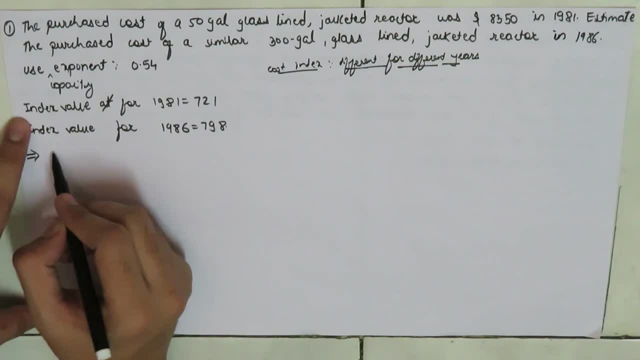 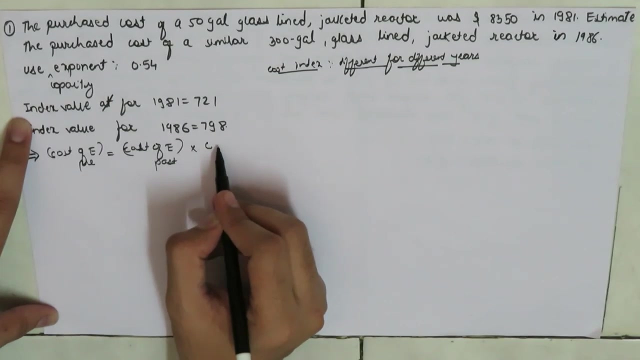 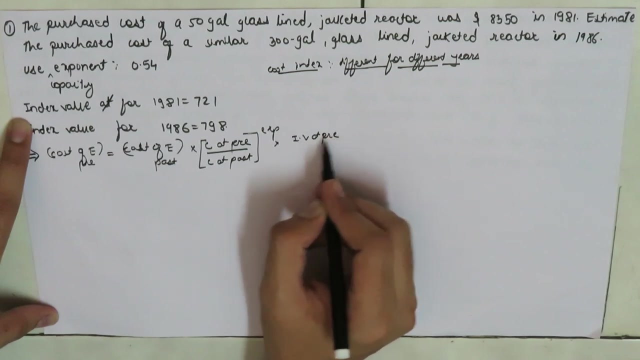 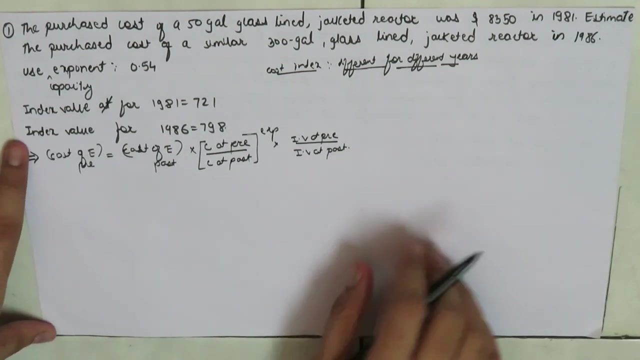 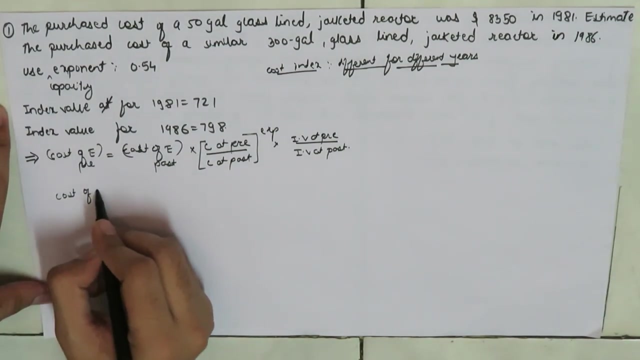 we are gonna use the basic expression. so the cost of equipment at present is equal to the cost of equipment at past, into capacity at present over capacity at present past. to the power, the capacity exponent times the index value at present divided by the index value at past. so from this given data we know that the cost of reactor 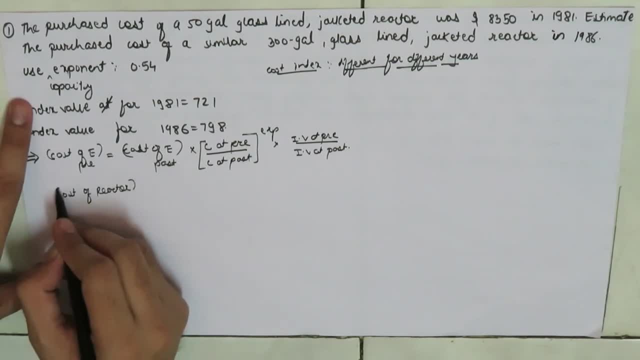 which capacity is 50 gallon, is eight thousand three fifty dollars- eighty five zero dollars in year 1981 and we need to find the cost of the same reactor in the year 1986 whose capacity is 300 gallons. so by making the use of this expression we can write the cost of reactor in the year. 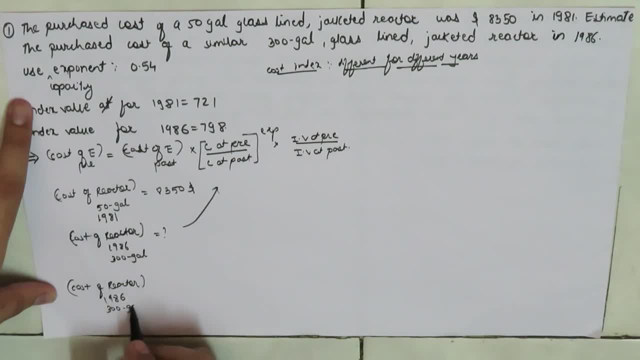 1986, whose capacity was 300 gallons, is equal to the cost of equipment at the past, means the cost of equipment in 1981 is eight, three, five zero dollars into. the capacity at present is 300 gallons over the capacity as past as 50 gallon. to the power the exponent is 0.54 times. 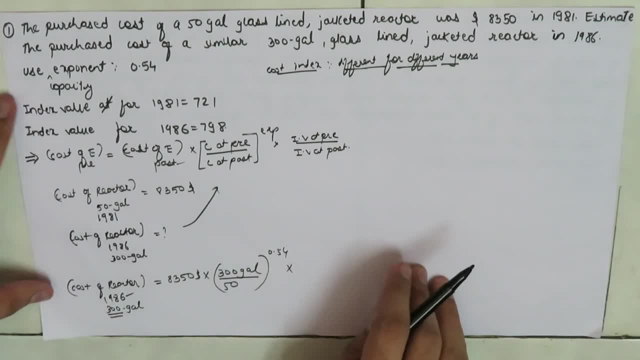 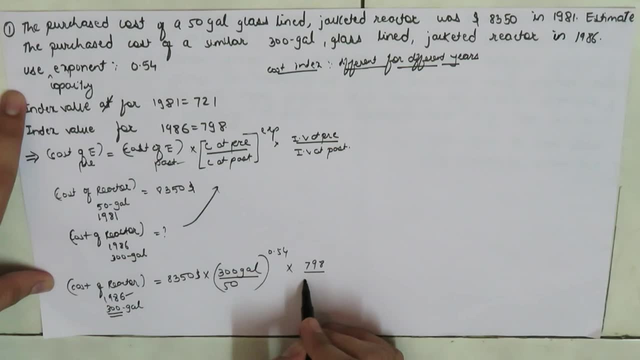 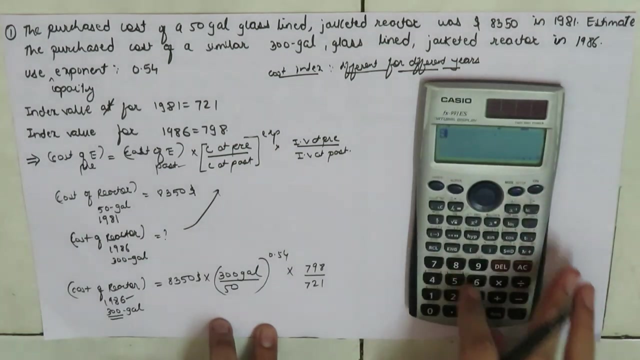 the index value at present means the index value in 1986 is going to be 798 or seven twenty one. so let me take out my calculator. so here we have 835, zero into into 300 by 15 to the power, 0.54 multiplied by 793 inch divided by 721, so the cost of the 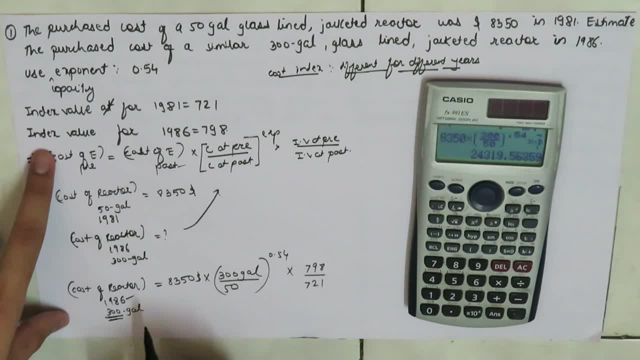 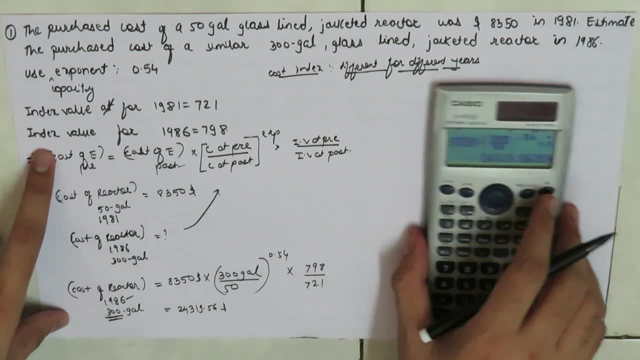 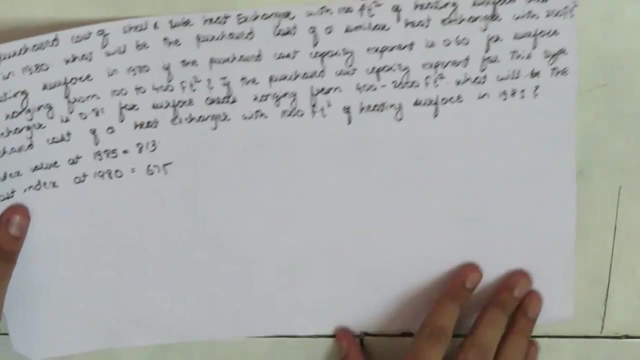 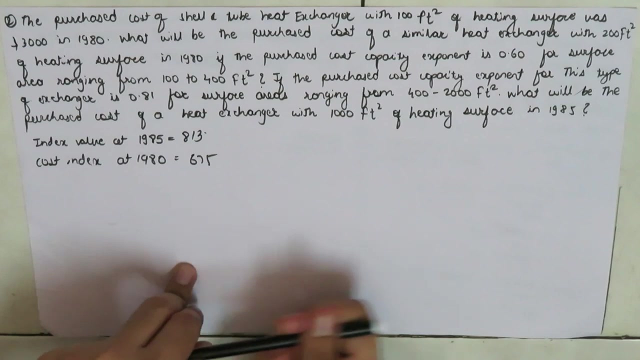 reactor in the year 1986 whose capacity is 300 gallon is equal to two, four, three, one, nine, point, five, six dollars. so let's take another example, and in this case we have the purchase cost of the cell and tube heat exchanger with 100 feet square. of the heating surface was dollar 3, 000 in the year 1980.. what will be the purchase cost of the similar heat exchanger with 200 feet seventeenth hour, even dollar? in this case we have the heat exchanger with BLACKCT Donc. certainly the cost of the cell is around 0.員 thousand percent of. almost the same level dollar heart rate, which says if you have electric and�� or two soi ную heat, the heat exchanger with hundred feet square of the heating- Cecilia hot, bar, Maxciano heat, exchritos, fromgg static- is as important value in year 1980, would you consider the cost of power? 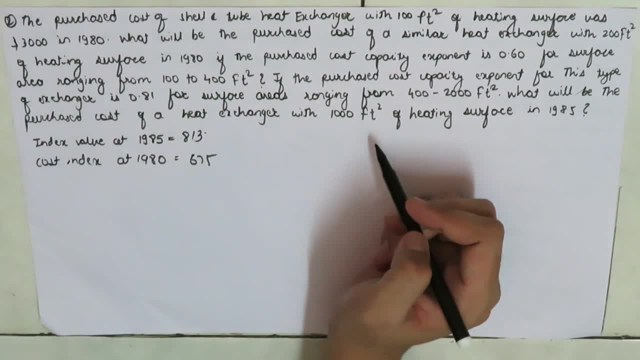 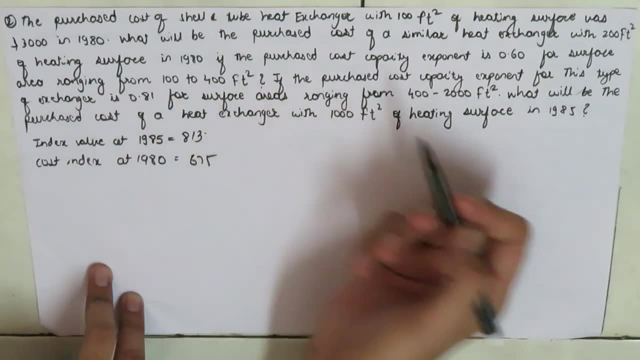 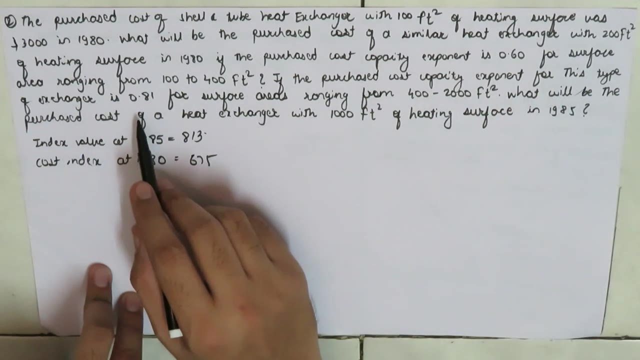 feet square of the heating surface in 1980, if the purchase cost capacity exponent is 0.60 for the surface area ranging from 100 to 400 feet square and if the purchase cost capacity exponent for this type of the heat exchanger is 0.81 for the surface area ranging. 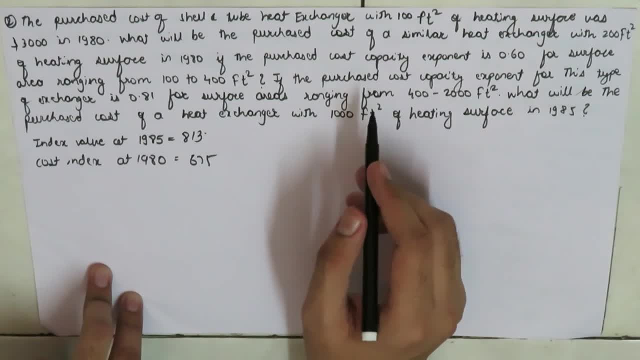 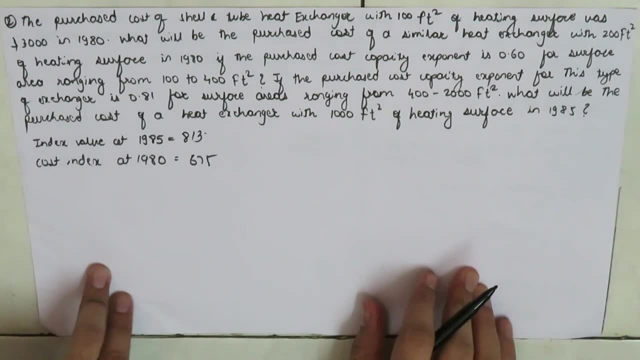 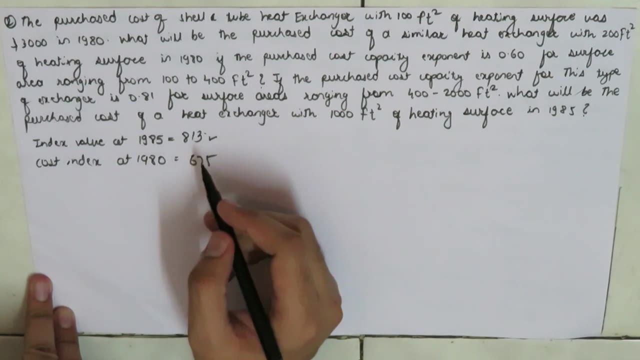 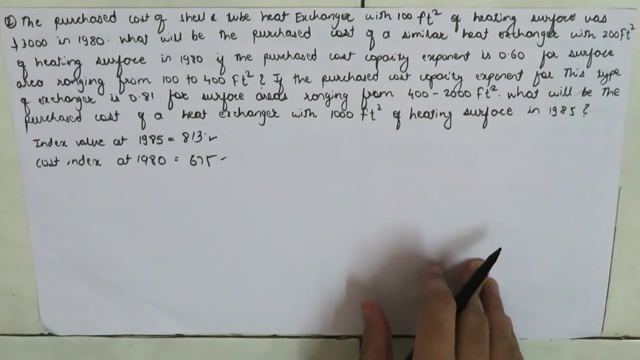 from 400 to 2000 feet square. then what will be the purchase cost of the heat exchanger with 1000 feet square of heating surface in 1985? and the given data is index value at 1985 is 813 and the cost index at the 1980 is 675. so here what we know, that the cost 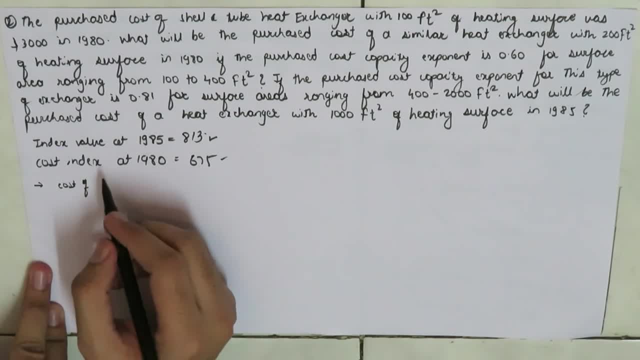 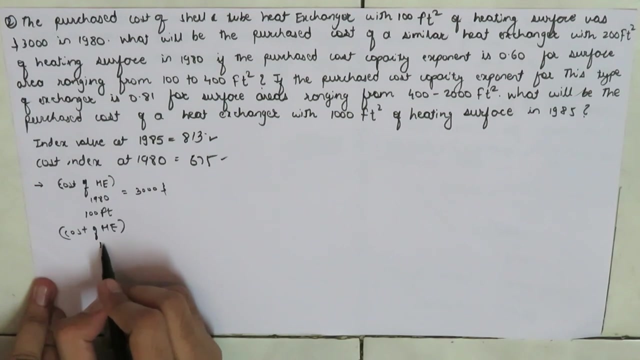 of heat exchanger in the year 1980, whose surface area was 100 feet square, is equal to $3000, and what will be the purchase cost of the similar heat exchanger? okay, so the cost of heat exchanger in the year 1980, whose surface area is 100 feet square, is equal to $3000, and the cost of heat exchanger 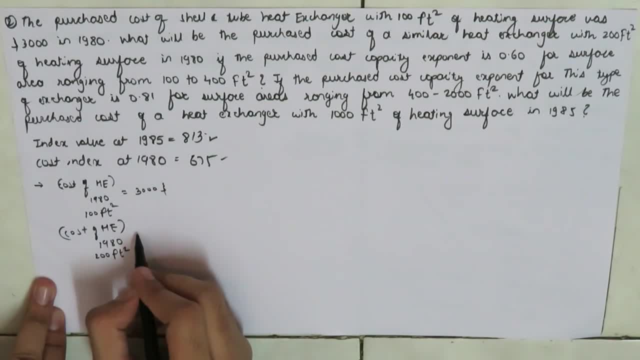 is 200 feet square. we need to find this and the exponent is 0.60 for the area ranging between 100 to 400, and here we are dealing with 100, from 200, from 100 to 200, and so we can use this exponent. so we know that the cost of heat exchanger in 1980, that is the cost of heat exchanger in 1980, which is 183, and this is not the cost of heat exchanger inộiusz. and if we look at the basic data, okay, we have one. we have the transform risk of this represents a quantity that goes back to 30 years and we know that the price of heat. 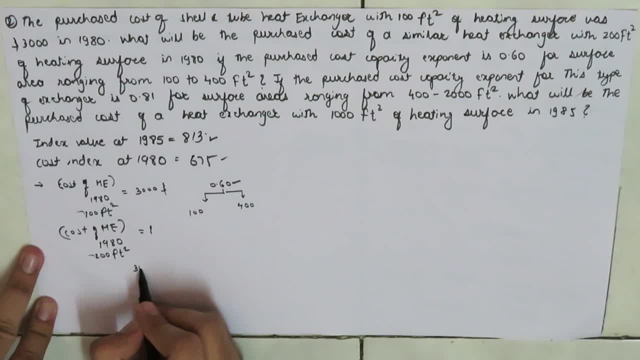 exchanger in 1980. okay, so what we're gonna do is here we have $3,000 times. the capacitor present is 200 feet square. that is the surface area divided by 100 feet square. to the power. our exponent is 0.60. the range of this exponent is from: 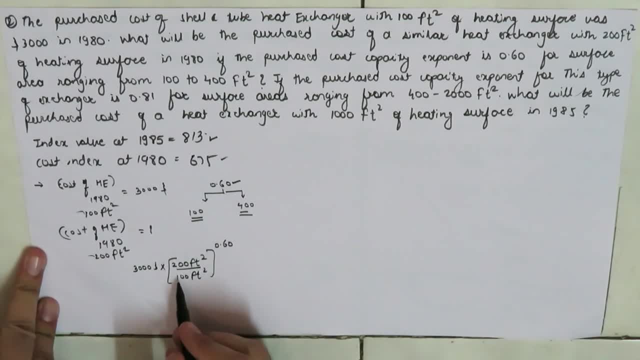 100 feet square to 400 feet square, and here we are dealing with from 100 feet square to 200 feet square, so we can wisely make use of this exponent. and do we need an index value for the same year? okay, if you need an index value for the. 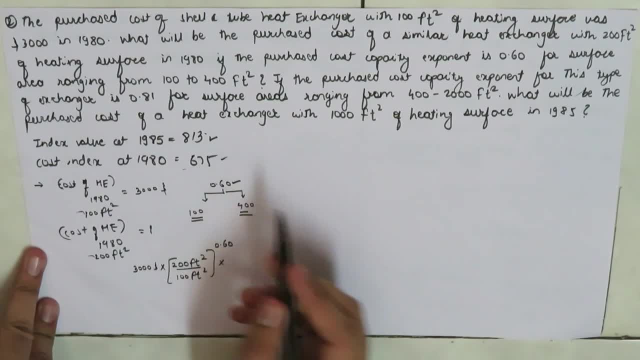 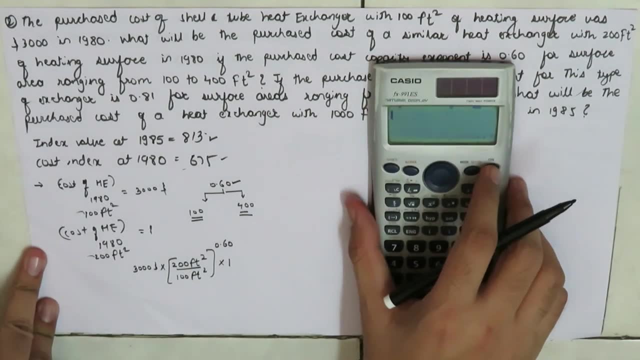 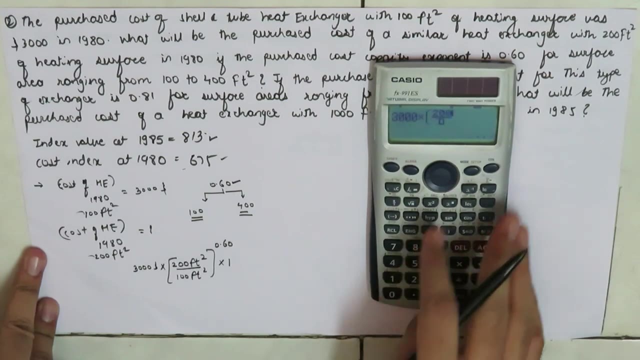 same year. they are gonna cancel out. so 675 over 675 is unity, so we are gonna take it as 1. so let me take out my calculator, for this is 3000 multiplied by 200 feet square, divided by 100 feet square to the power, 0.60 is four five, four, seven point one. 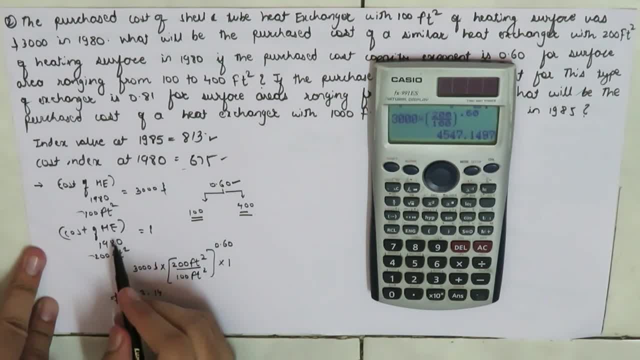 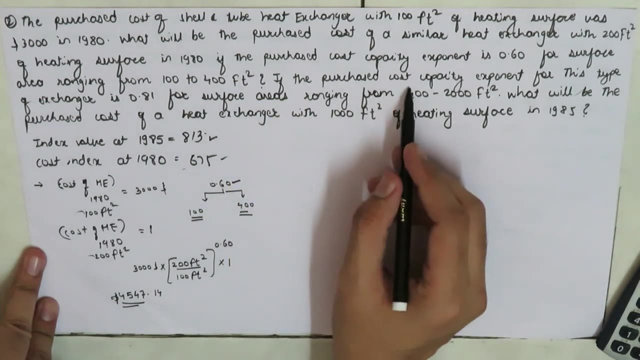 four dollars. so the cost of the heat exchanger in the year 1980, whose surface area is 200 feet square, is four, five, four, seven point one, four dollars and further. what we need to do is in the purchase cost of the capacity exponent for this type of. 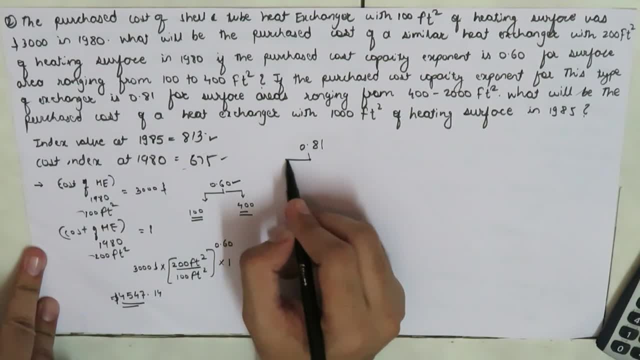 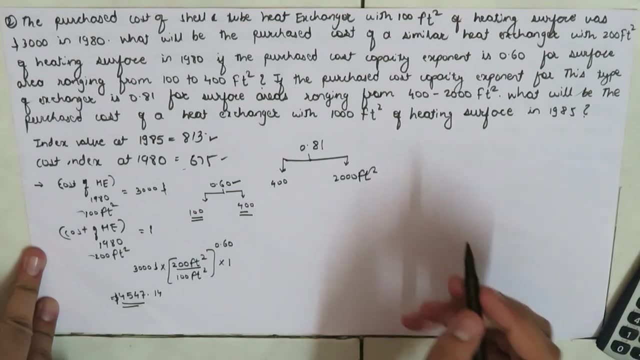 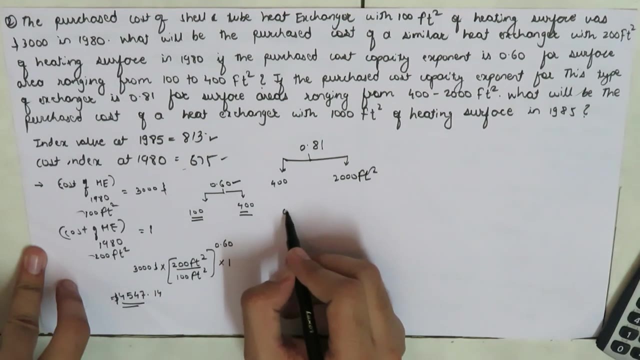 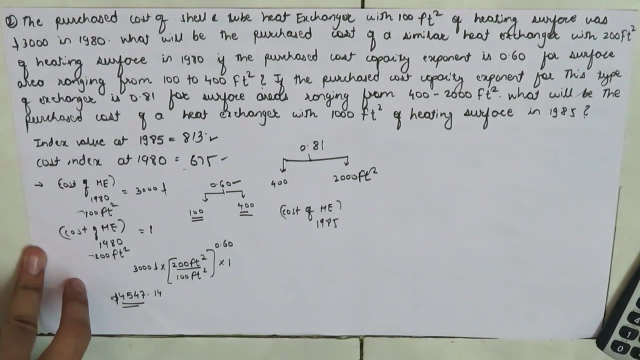 heat exchangers, zero point 81 for the surface area which is ranging between 400 feet square to two thousand feet square. then what we did? the purchase cost of the heat exchanger with thousand feet square, feeding surfaces, hitting surface. so we need to find the cost of heat exchanger in the year 1985, whose 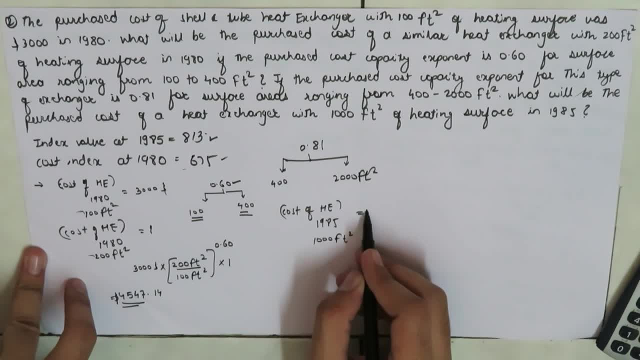 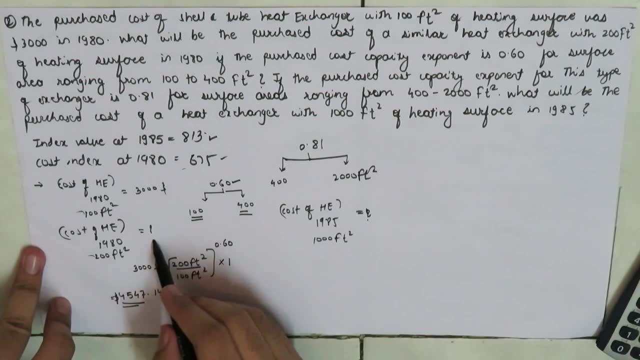 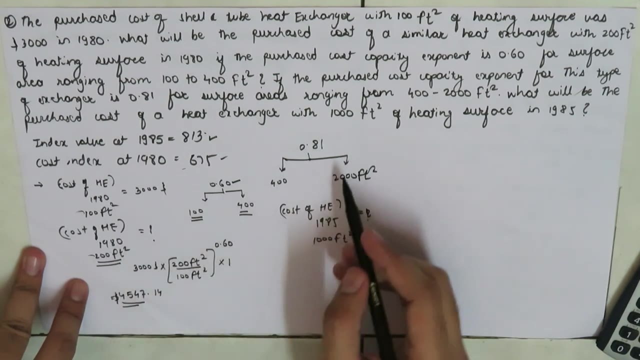 area is thousand feet square, equal to question mark. so here in this case, if you make use of this value, but this value is calculated for 200 feet square heading surface area and the exponent is point 81 for the surface area which is a ranging between 400 to- 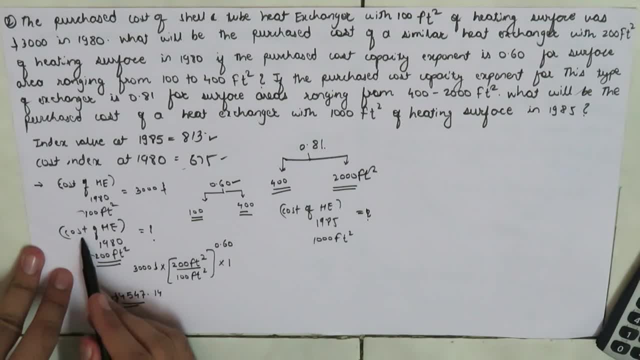 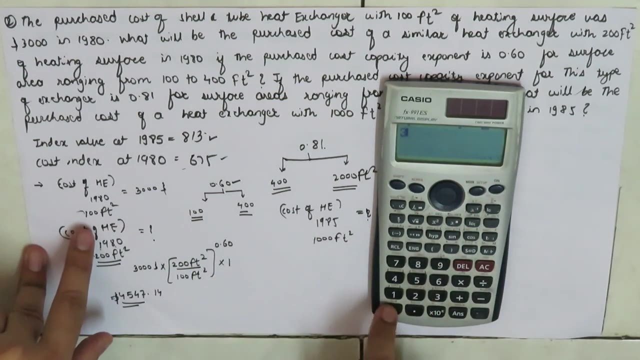 2000. so what we need to do is we need to calculate the cost of heat exchanger in 1980 whose surface area is 400 feet square. so the cost of heat exchanger in 1980, whose surface it is 400 feet square, can be given as the cost of heat. 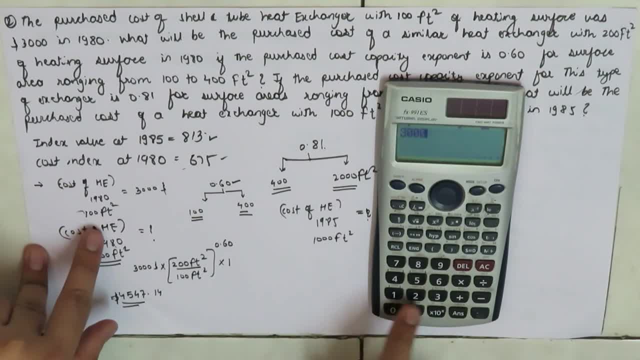 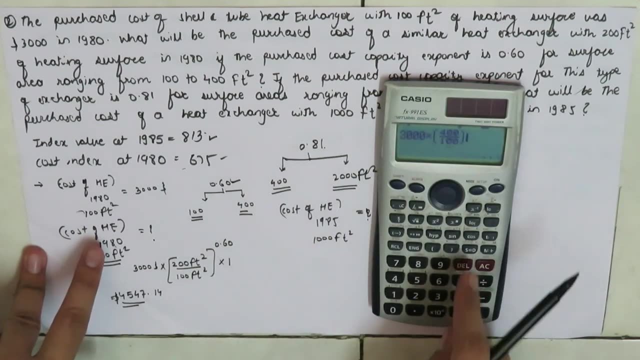 exchanger in 1980, whose surface it is 100 feet square times 400 over hundred, and as we are dealing with the surface area between 100 to 400, we can make use of the exponent. so this is to the power point, sex. and as we are dealing with the same, 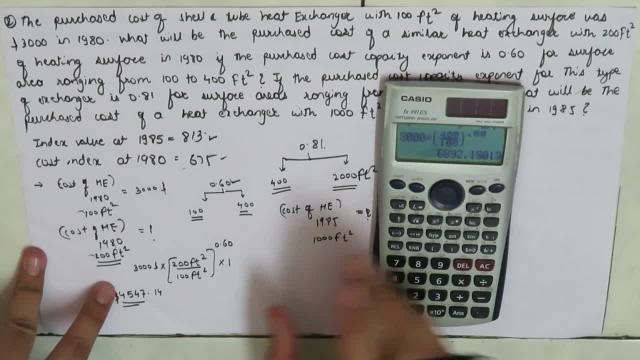 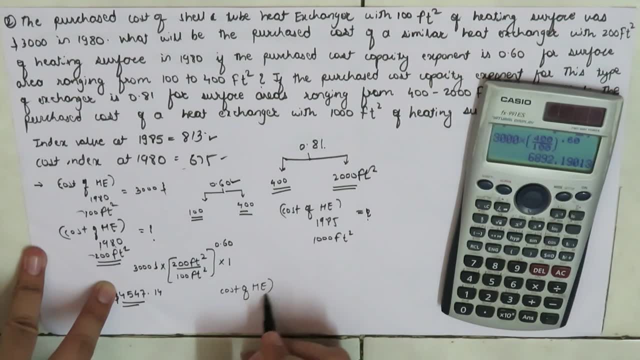 year. so this will in this value will get cancelled, and the cost of heat exchanger in nineteen, eighty five for the cost of heat exchanger in 1980, sorry would. surface area is 400 feet. square is equal to six, eight, nine, two point one ninety. 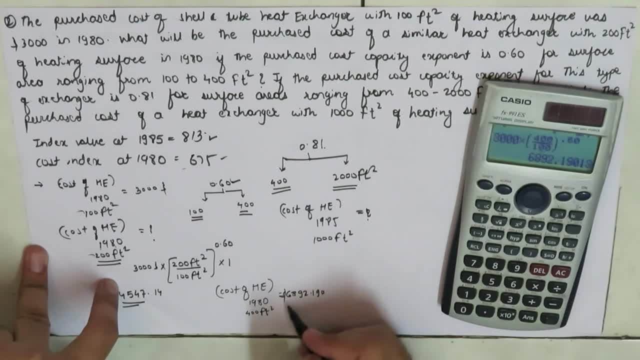 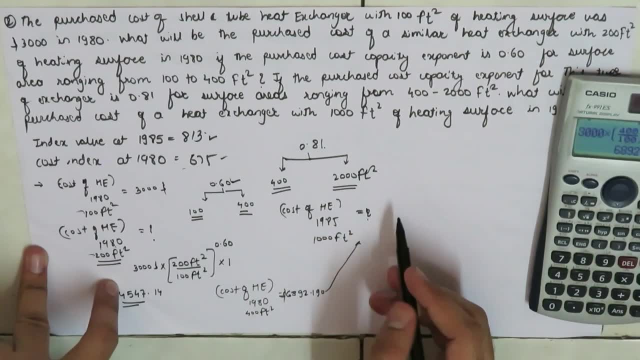 dollars. so we are going to make this value, we are going to put this value in this equation to calculate the cost of heat exchanger in 1985. so this will be equal to six, eight, nine, two point one ninety dollars times thousand feet square over 400 feet square, to the power exponent as: 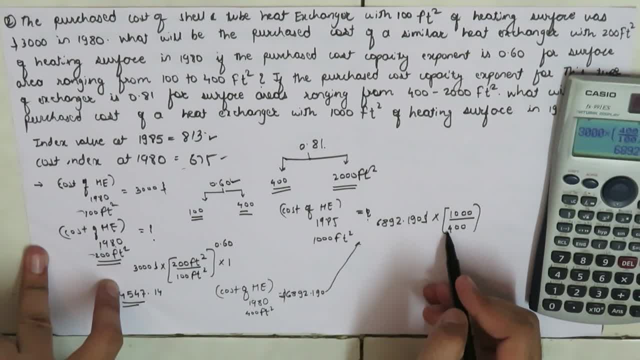 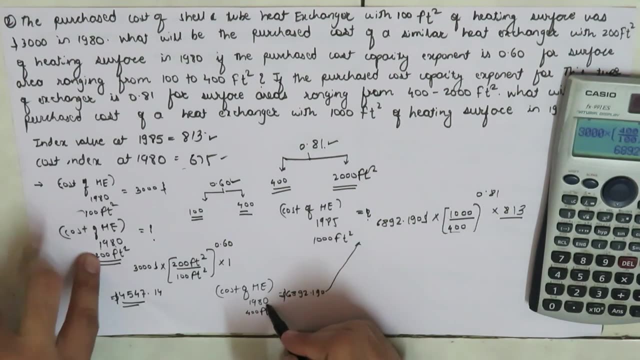 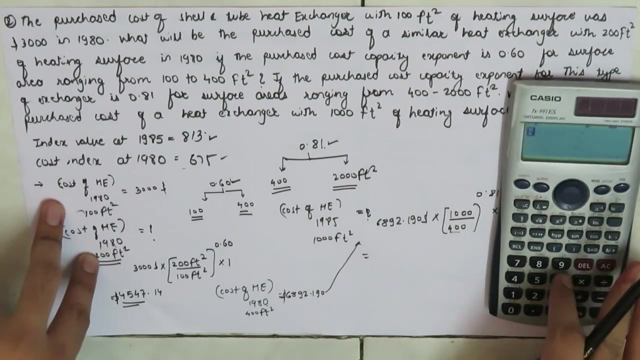 we are dealing with the heating surface area between 400 to 1000, so we can make the use of this exponent, so 0.81 into index value. at present is index value at 1985 this is 813 over. the index value at 1980 is 675. so this will be our six, eight, nine, two point one, ninety times. 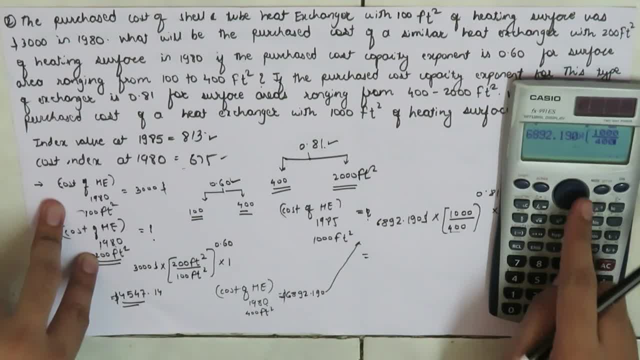 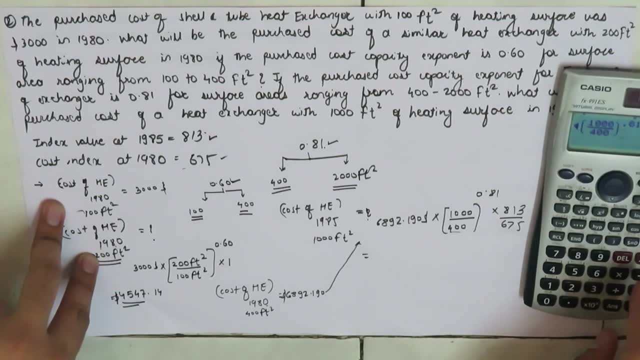 thousand by 400 to the power point, 81 times 813 over 675. so this is going to be equal to 17437.14. so the cost of the heat exchanger in the year 1985 whose heating surface area is 1000 feet square. 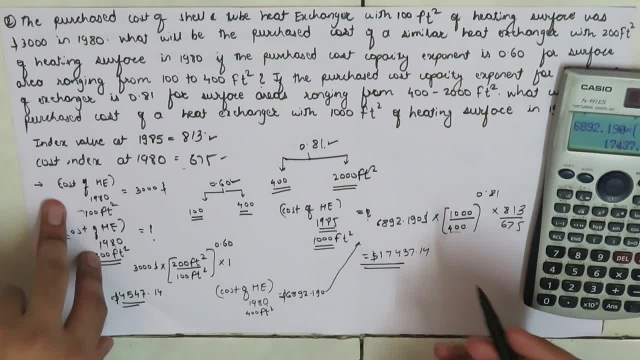 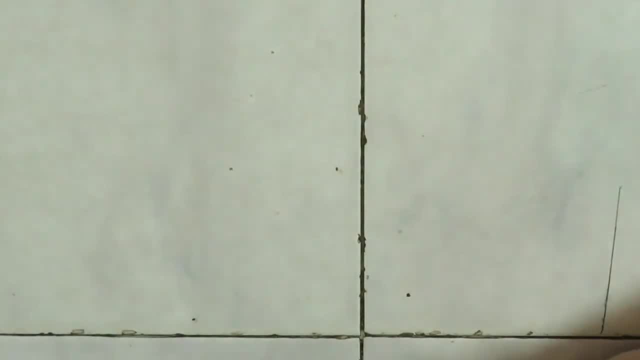 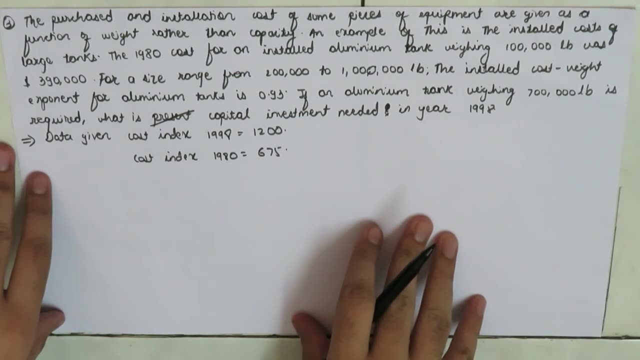 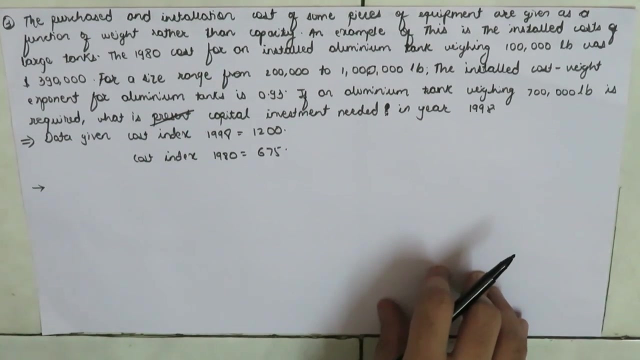 is equal to 17437.14 dollars. but in some cases, instead of dealing with the areas, we will deal with the weight of the reactor and we have the problem which is dependent on the weight of the reactor. so here we have our question: the purchased and installation cost of some pieces of equipment. 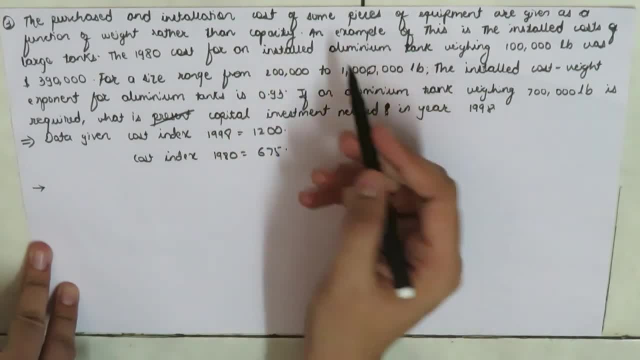 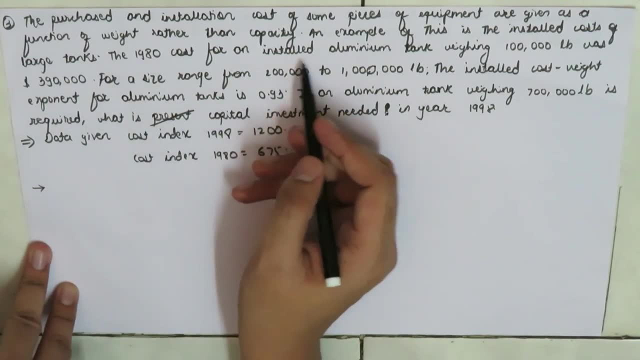 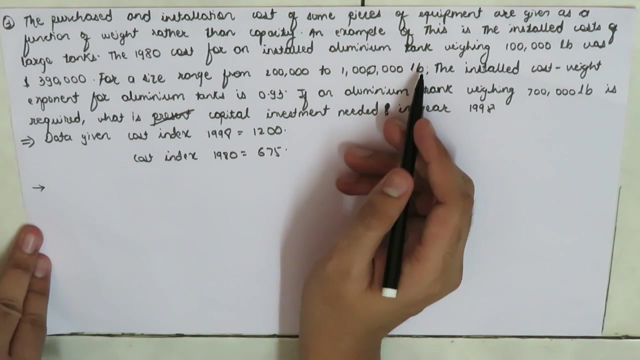 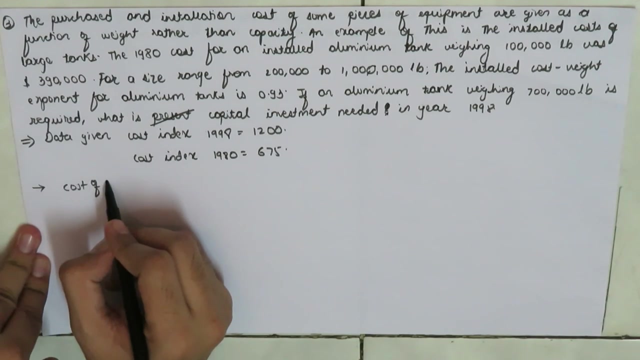 are given as the function of weight rather than a capacity. an example of this is installed cost of. the last times in 1980 the cost of installed aluminium tank weighing 10 to the 100 times 10 to the power, 3 pound was 390 into 10 to the power, 3 dollars. so here we have the cost of. let's call. this our tank. okay, cost of tank in the year 1980 whose weight was 100 into 10 to the power 3 pounds was equal to dollar 390, triple zero for the size range from 200 into 10 to the power 3 to 10 to the power, 6 pound the installed cost. 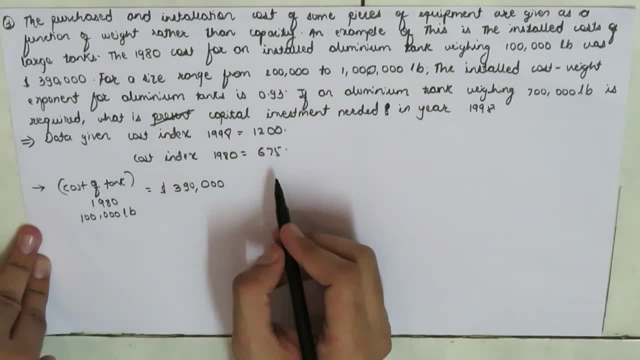 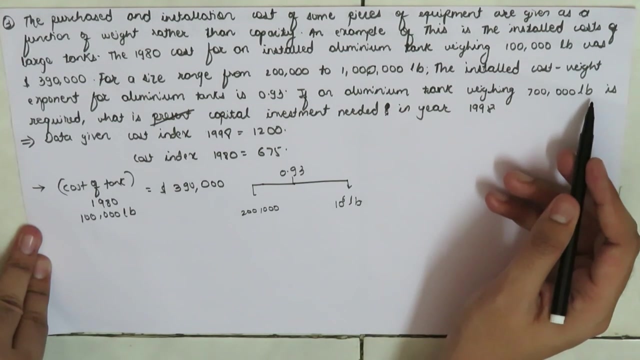 weight exponent for the aluminum tank is 0.93. so the exponent is 0.93 for the weight, which is ranging between 200 into 10 to the power 3 to 10 to the power 6 pound. and if an aluminum tank weighing 700 into 10 to the power 3 pound is required, then what is the 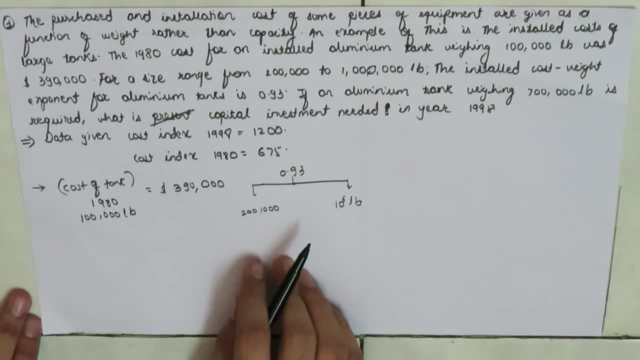 capital investment needed in the year 1998.. so we need to find the cost of tank in the year 1998, whose weight is 700, into 10 to the power 3 pound. so this is equal to the cost of equipment at the past means. 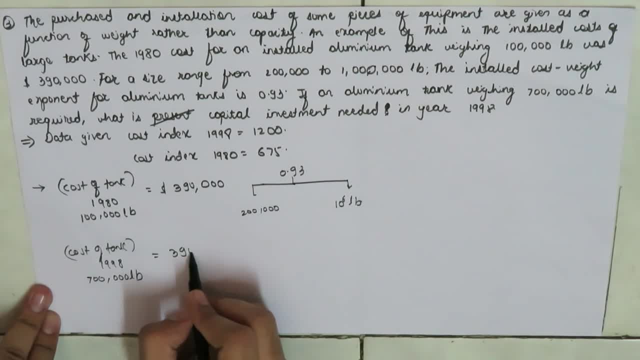 the cost of the tank in 1980, so this is 390, triple zero times the weight of the tank at present. this is 700 into 10, to the power 3 pound divided by the weight of the tank in past, so this is 100. 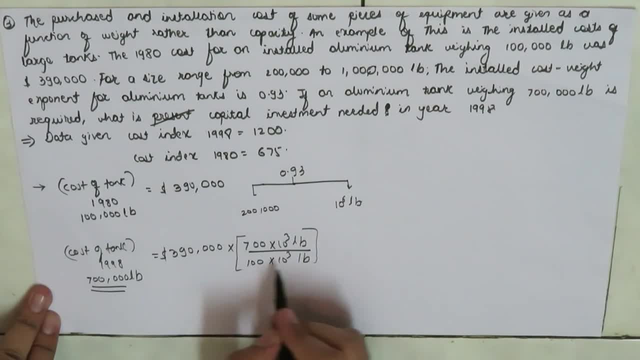 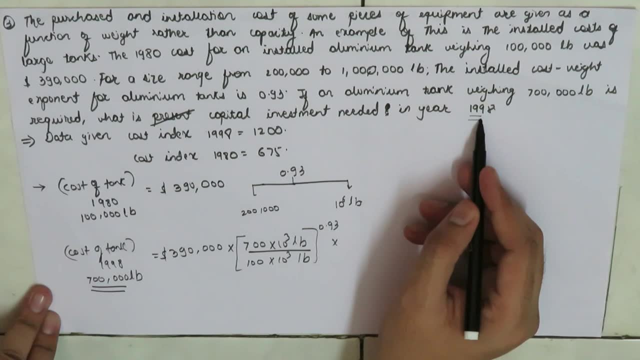 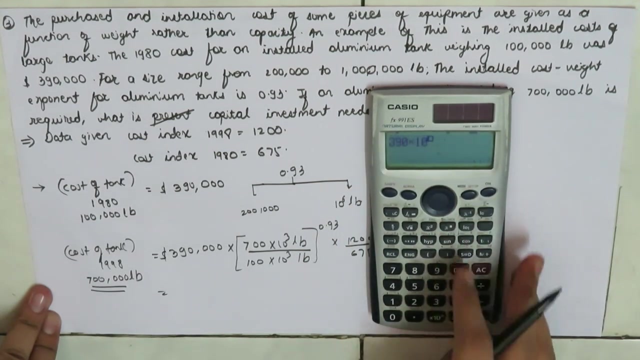 into 10 to the power 3 pound, the second power and the exponent is 0.93 into the index value� out. the present, that is, the index value at 1968, is 1200 over six 75, which is equal to 390 into 10 to the power 3 multiplied by 700 over. 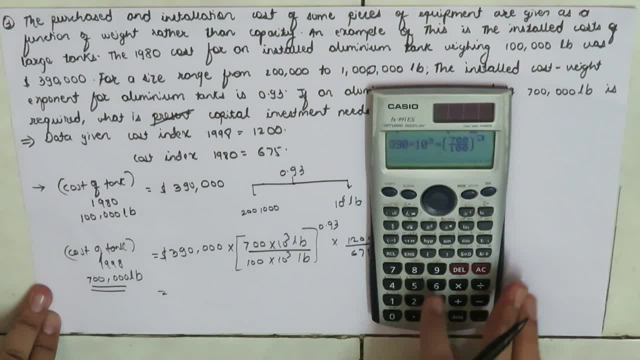 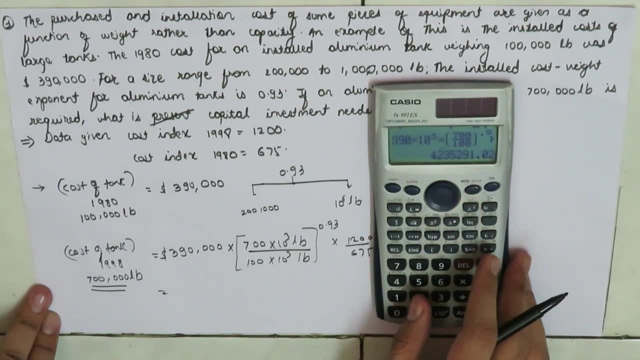 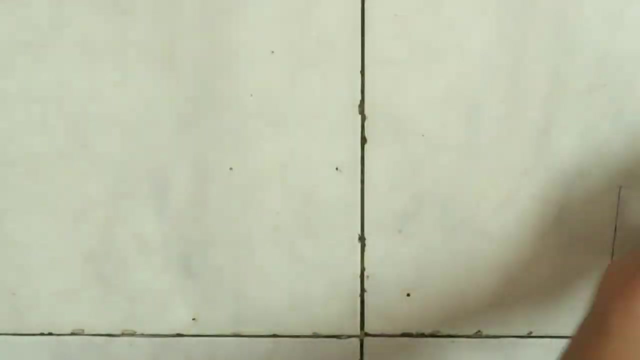 hundred to the power point 93, multiplied by 1, 2, double 0, divided by 675. so here the cost of the tank in 1998, whose weight was 700, into 10 to the power, 3 pound, is 4, 2, 3, 5, 2, 9, 1 point 0, 2 dollars. so let's take another example where the 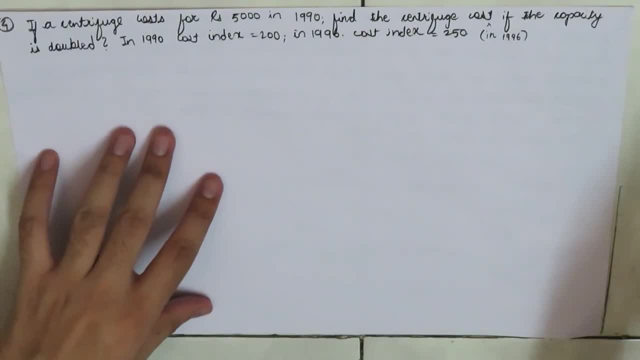 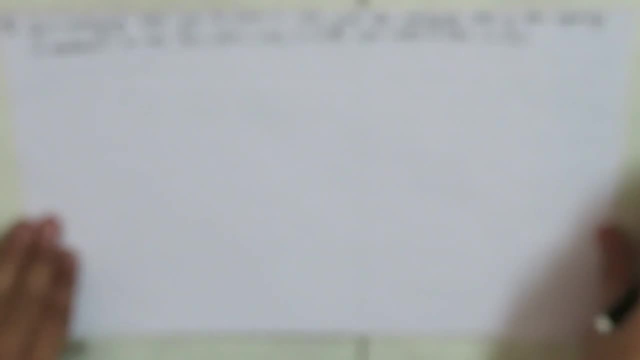 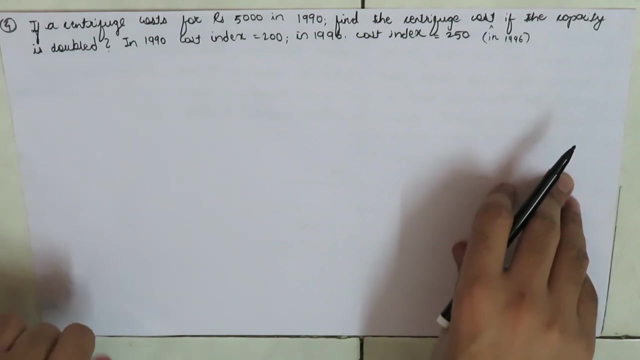 capacity exponent is not mentioned. so when the capacidad exponent is not mention be directly mean we are directly going to make the use of the 6-by-10 factor 2. so here's an example which is dependent upon the use of six by ten factor rule. if a centrifuge cost. 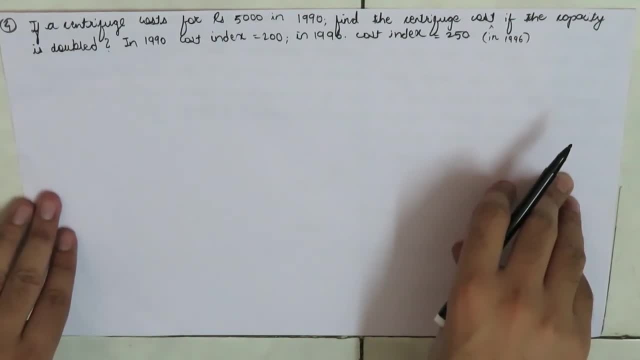 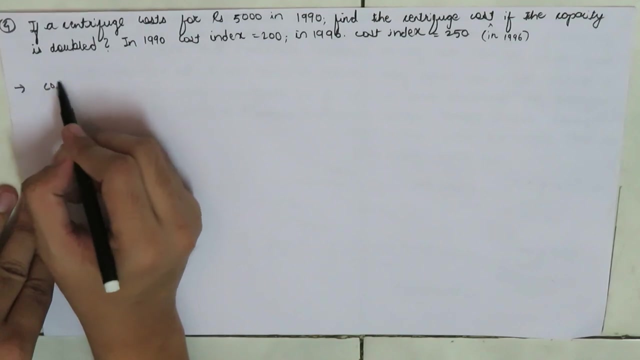 for rupees 5000 in 1990. find the centrifuge cost in the if the capacity is double. in 1990 the cost index is 200 and in 1996 the cost index is 250. so we know that the cost of equipment that is our centrifuge, sure in the year 1996 is.